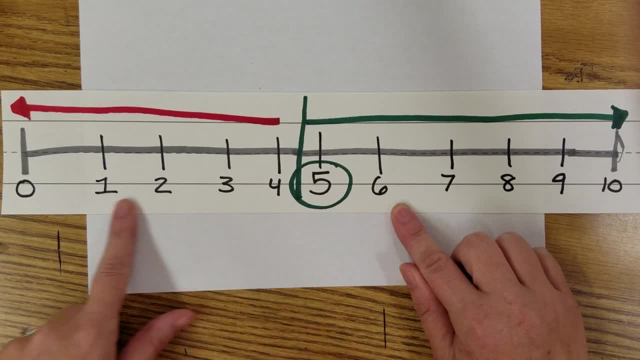 Okay. so 0,, 1,, 2,, 3, and 4 are going to tell you to stay Okay. 5,, 6,, 7,, 8, and 9 are going to give you the green light. 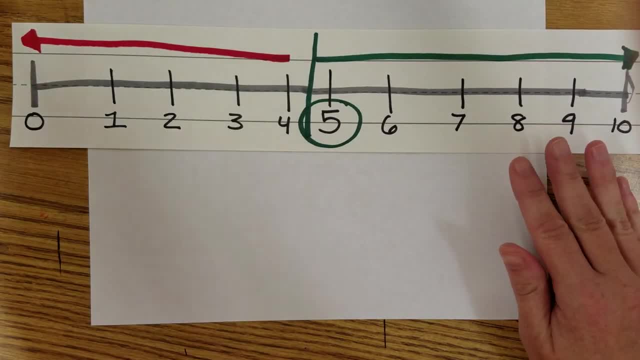 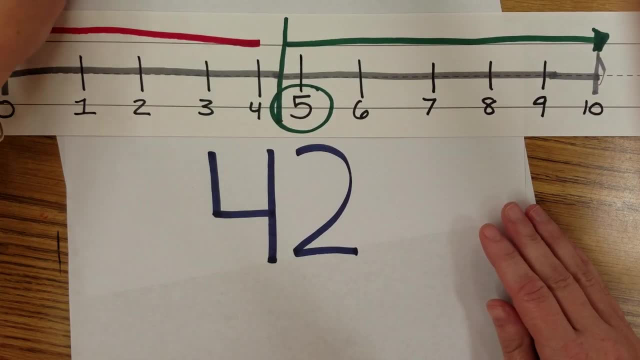 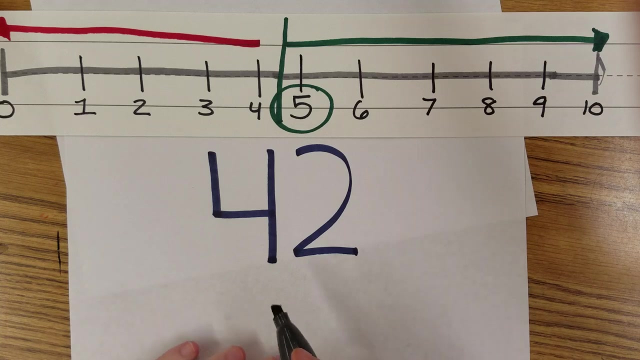 and they're going to tell you to go up to the next 10.. So we're going to practice that. Okay, our number here is 42. So the first thing we need to do is figure out which number is in the 10's place value. 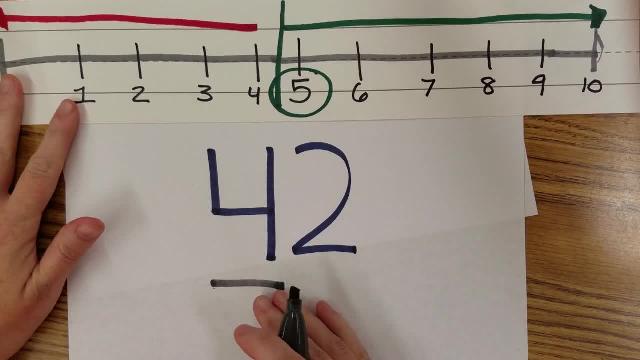 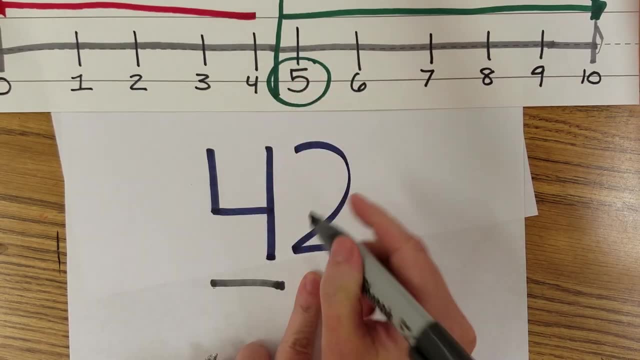 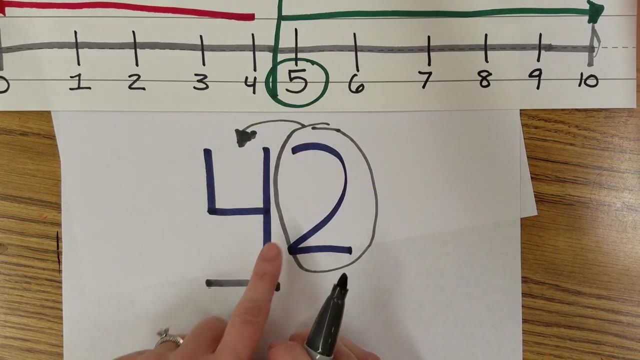 So for this one, the 4 is in the 10's place value. That means that the 2,, which is in the 1's place value, is the boss. This number is the boss of this number and it's going to tell it what to do. 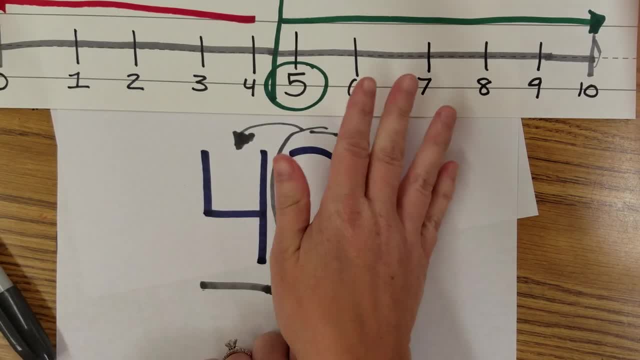 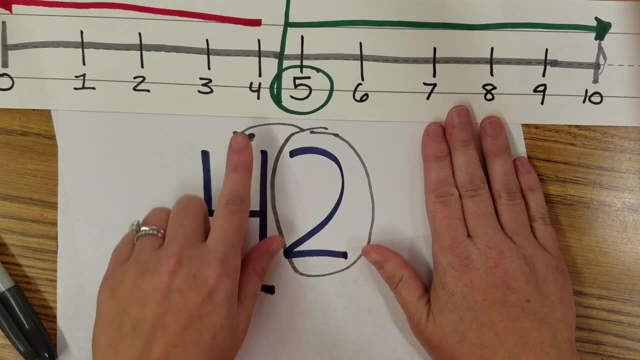 So if whatever number is in the 1's place value- if it's 0,, 1,, 2,, 3, or 4, it's going to tell it to stay at 4.. If the one in the 1's place value is 5,, 6,, 7,, 8, or 9,, 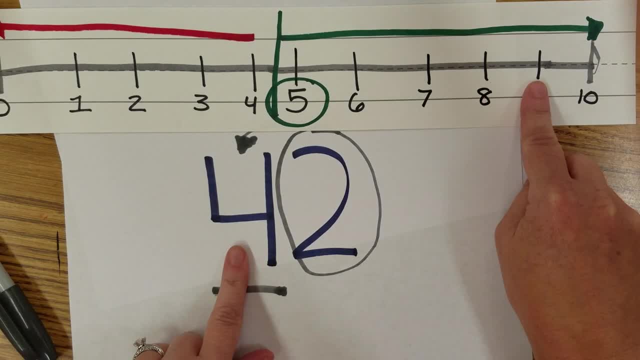 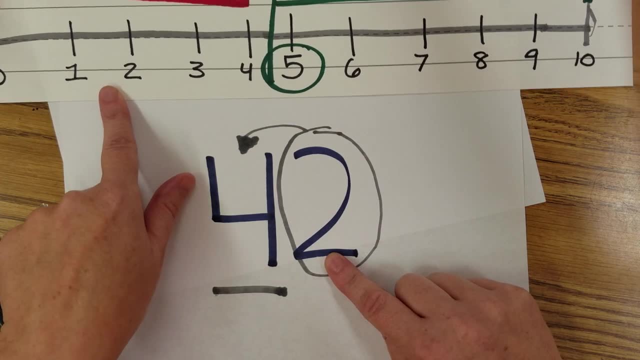 it's going to tell you to go ahead to the next 10.. We can see that the 2 is a small number and it's going to tell you to stay at the 10's. This one will stay. Your 10 is going to stay at 4.. 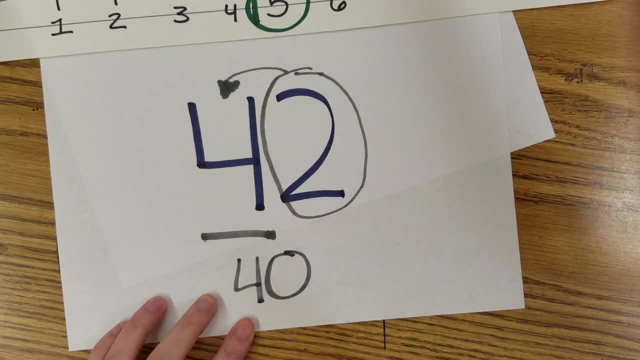 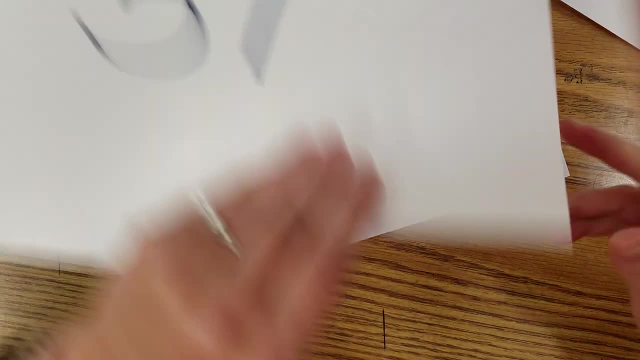 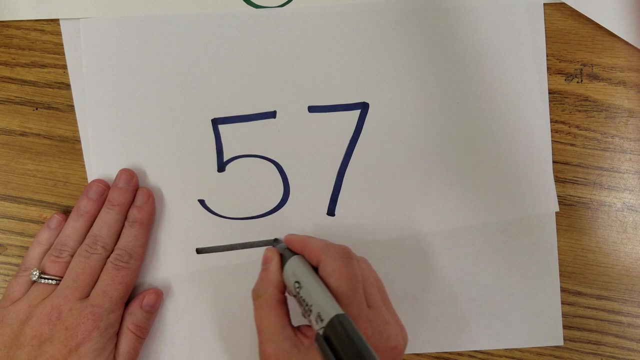 Now you put the 0 in the 1's and you're going to take it to 40. So 42 is going to round to 40.. Okay, let's try another one. This one is number 57.. So again, we look at the one in the 10's, which is the 5.. 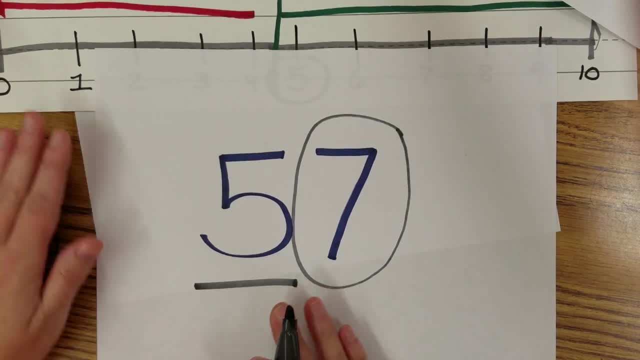 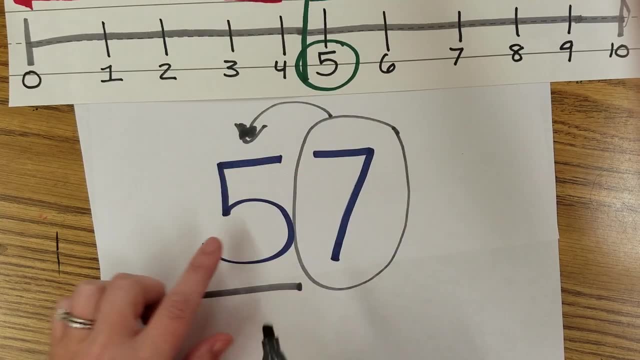 The digit in the 1's place value is the boss, though That one tells it what to do. Okay, so the 7 is going to tell the 5 what to do, Because the 7 is a big number. you can see it's on this side of our number line. 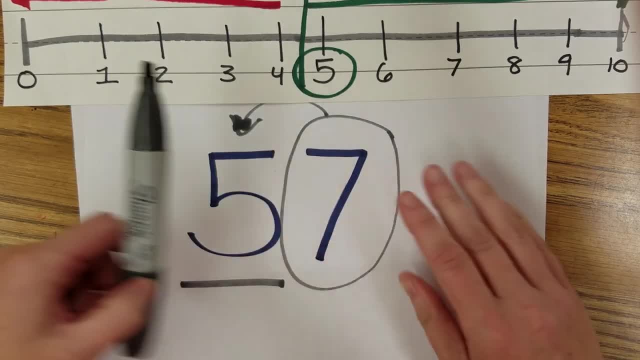 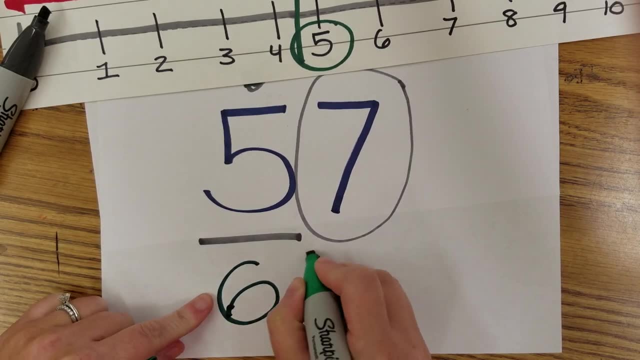 it's going to tell the 5 to go up to the next 10, to add one, 10.. So that gave it the green light 57,. this goes up to 6,. it's going to be closer to 60..